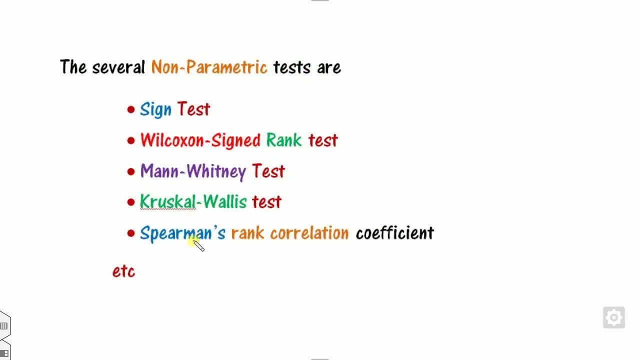 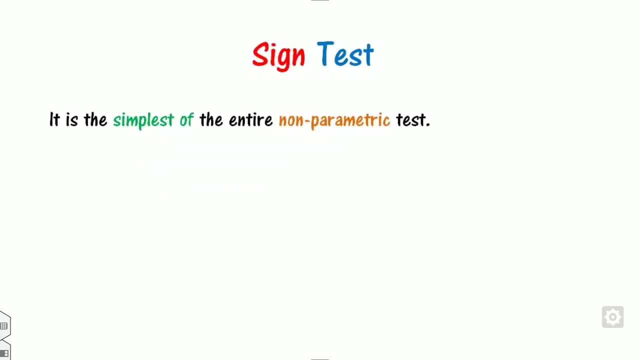 Sine test: Wilkerson, Mann-Whitney, Crucial and the rank correlation, etc. We will cover this one by one And in this lecture we will start with the first, that is a sine test. So first of all, 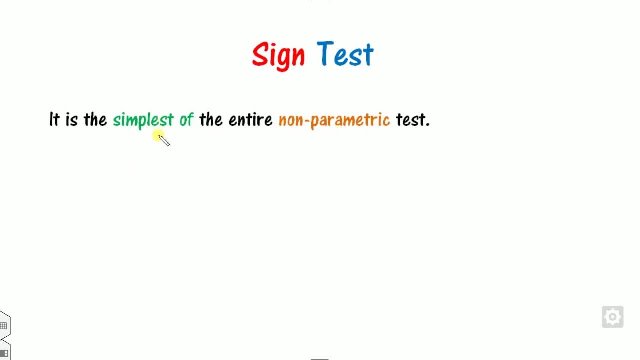 this is one of the simplest test of the non-parametric. As the name suggests, that is a sine. What is the meaning of the sine is That is a plus or minus. So it is based on the sine of the test rather than the exact magnitude. If I say my numbers are say 41,, 39 and so on. So it is not. 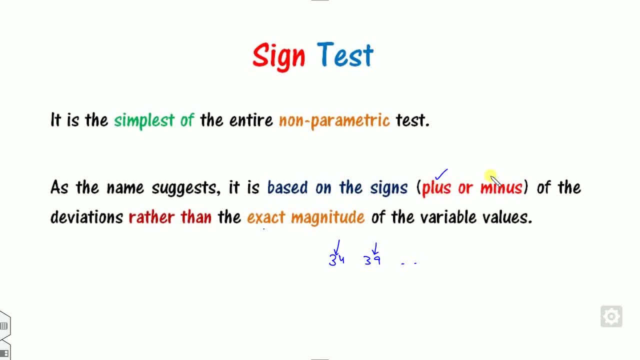 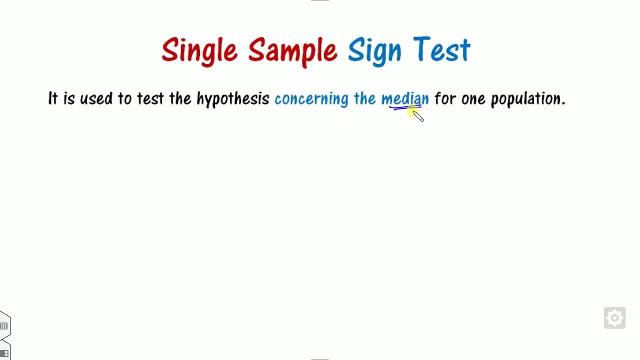 depending upon these 34 and 39. It is only depending upon their sines plus and minus. So this test is basically used for concerning the medians for the one population. So we are discussed about the single sample, So it is discussed about the median and we use throughout the lecture as 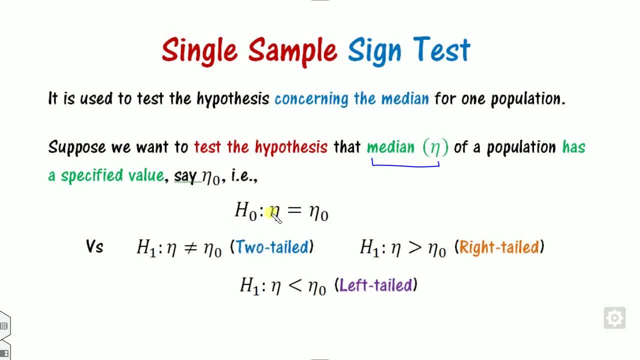 median as my eta. So this is a symbol. So so my test testing of hypothesis is: we will check that whether the median is some, this eta 0 is some specified value. That is, we will check that whether the median of the population is. 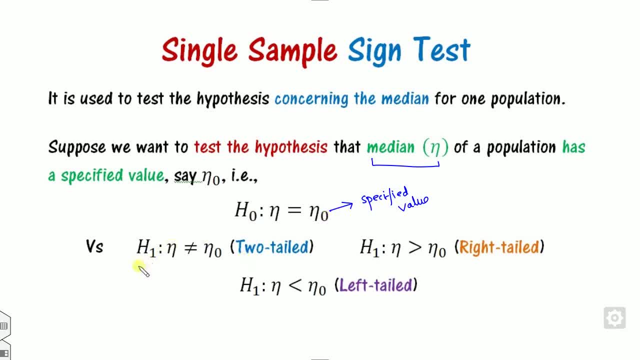 equal to eta 0 or not, against some alternative. So this is my alternative hypothesis. So that alternative hypothesis is either of the two tail or the one tail, which is categorized as right or left. Now how to find how to apply the sign test. So assume that there are the sample size of 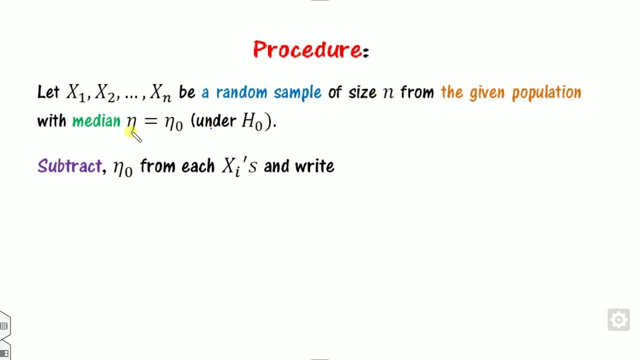 n, which is given from the population, and this is under h. 0 is my eta is no. So how you? what is the procedure is? you can subtract this eta node from the each observations and what is the meaning is if I say my x i's are this, say 43,, 29,, 53 and so on, and I will want to check eta as my say 43. 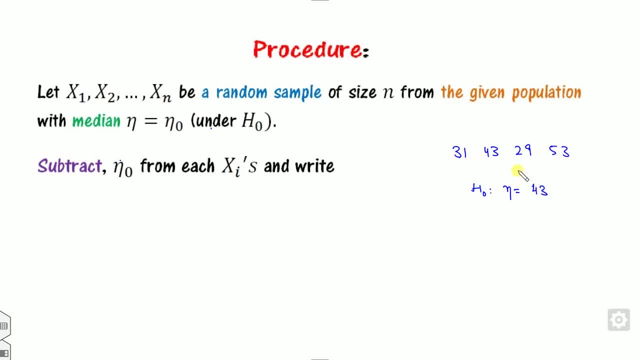 So we will subtract 43 from the each, 31 minus 43 and each and we can write only as their plus if the deviation is positive. negative if deviation negative. 0 if it is 0.. For example, in this case, what is the deviation is negative, So we can write minus, this is 0. This is negative. The 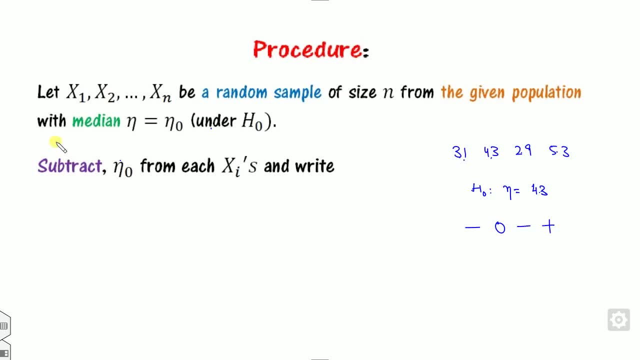 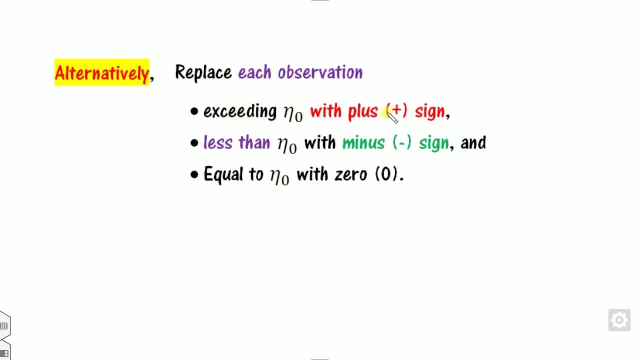 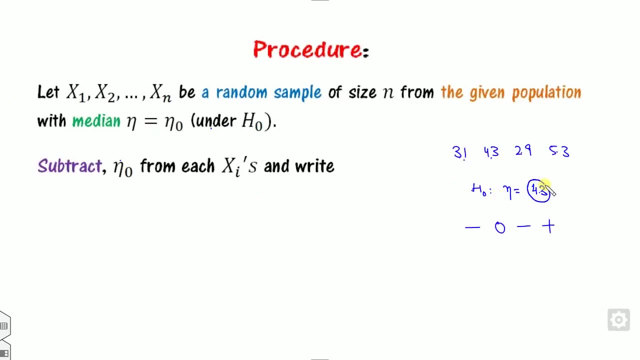 deviation is positive. We are not focused on the value, So this is there. Otherwise, you can also use this notation. You can put the plus sign which are exceed this like. say this: in this case, you can see that which number which are greater than of the 63, only this we can write as a. 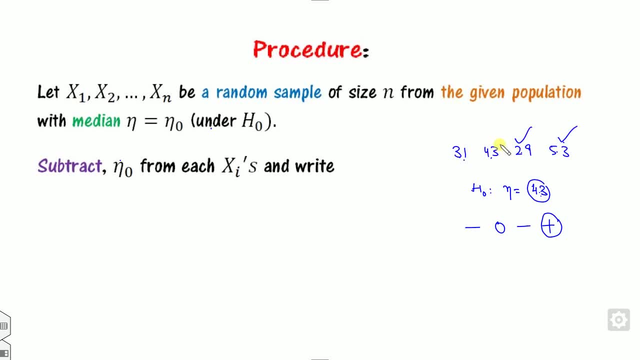 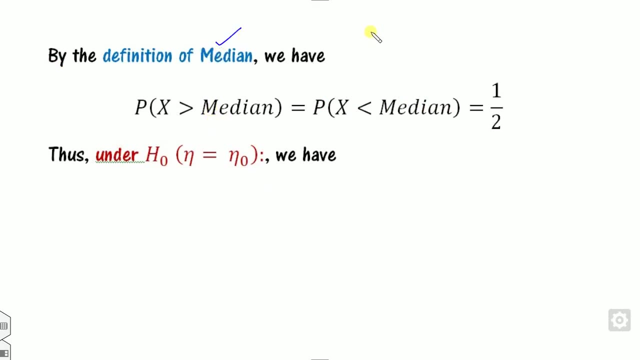 plus sign which number which are less than of the 43, these two, So we take a negative sign, and which numbers are equal, we will put as a 0. So you can use either of this notation or this. Now, since what is the definition of the median? since the sign test is working on the median. So what is? 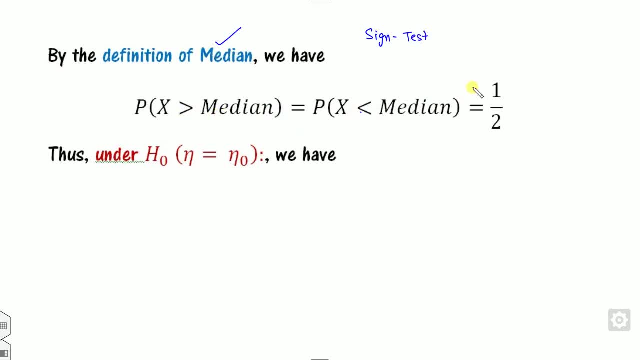 the definition of the median is it's the position which divides the series into the equal parts. So what is the meaning of that? under this h0, what we have- So we have median- is nothing but my eta 0. So this is nothing but half. So we will check that h0 is true. then the number of the positive. 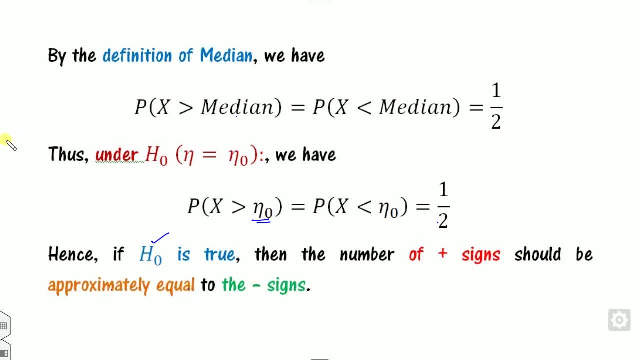 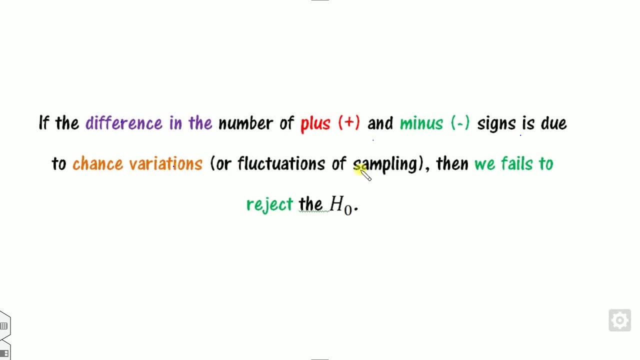 sign should be approximately equal to the negative sign. So look at that. So if this difference, our task is to check that the number of the positive and the number of the negative signs are equal- If the difference is due to the chance or fluctuation of the sampling, then we will fail to reject the h0, that is, we will. we. 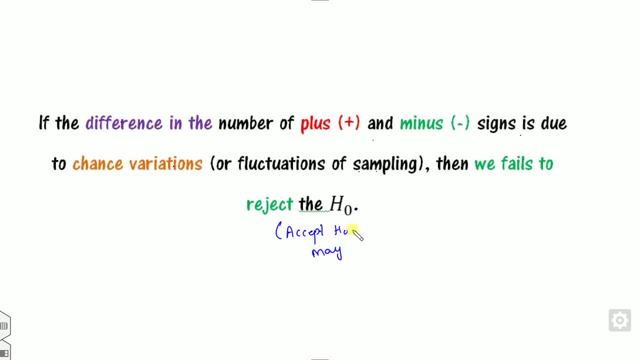 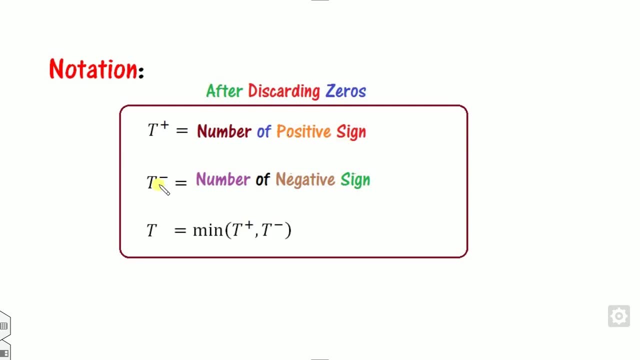 may accept the h0.. That is the meaning of it. So what is that? So look at the notation. we will define T- positive number of the positive signs, T negative number of the negative signs, and capital T as the minimum. This is computed only after discarding 0.. What is the meaning of? 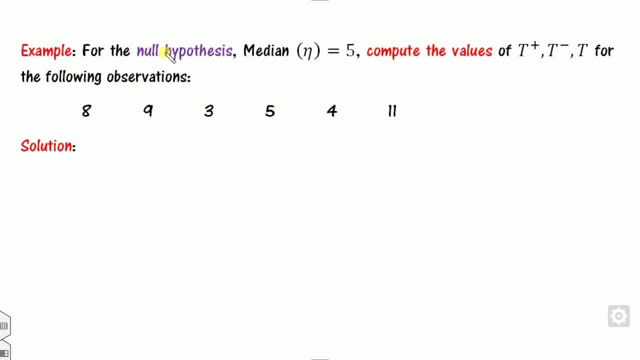 this is. look at this example. So, first of all, what is a null hypothesis is h0, is my. here You have to compute T positive, T negative and T for the following information. So what you can do is subtract 5 from the each of the numbers and write their sign. For example, 8 minus 5 is a positive. 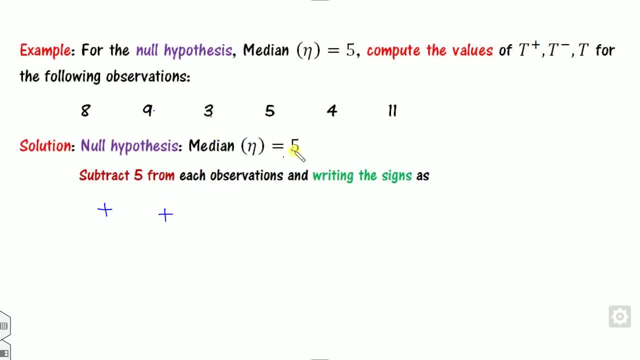 9 minus 5 again is a positive. 3 minus 5 is a negative. 5 minus 5 is 0,. 4 minus 5 is negative. 11 minus 5 is positive. Now you can compute the positive signs. How many positive signs are there? 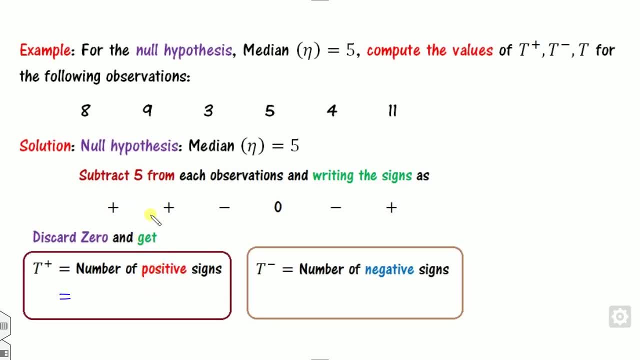 3.. So number of the positive signs, how many positive signs? 3. Okay, how many negative signs are? 2.. Then you can define the capital T as minimum of T positive and T negative. So you will get as a 2.. So this is a way you can compute. 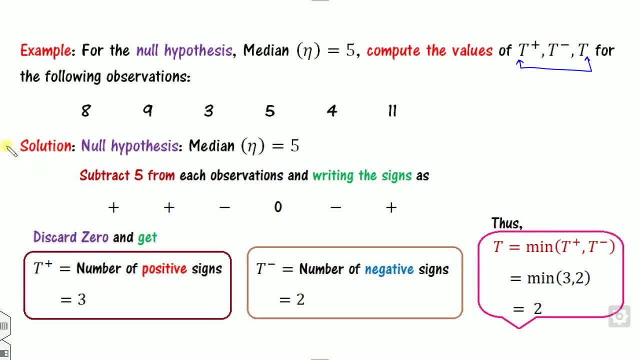 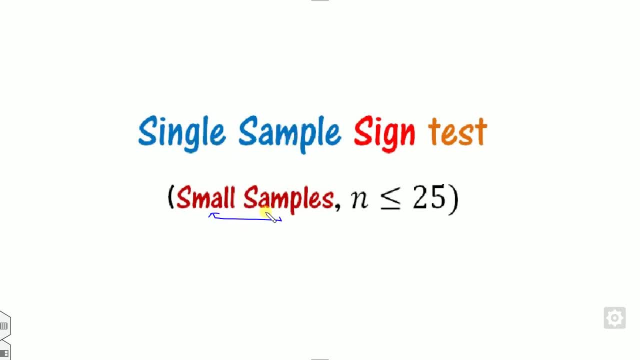 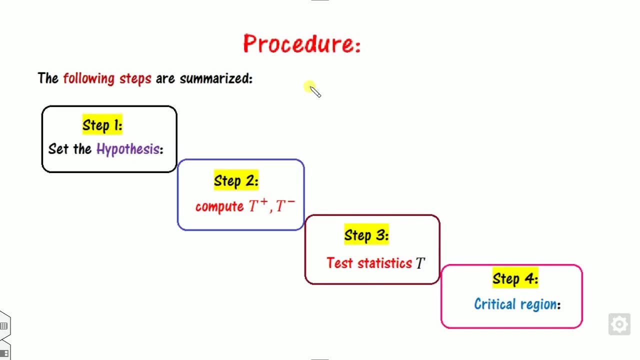 T positive, T negative and T in each of the example. So let us start with a single sample for the small sample. So when the sample is size is less than of the 25, then we call as the small sample for the sign test. So what is the procedure? is that we can compute this in the 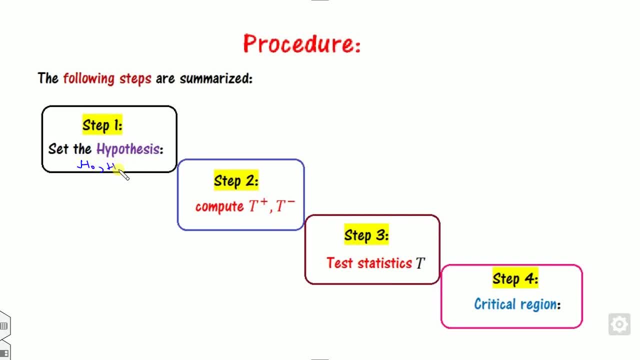 first step. So what is the procedure? is that we can compute this in the first step. We will define the hypothesis, that is, H0, H1.. We will compute T- positive and T negative, as we discussed in the last example How you compute the T, as This is nothing but my minimum of positive and 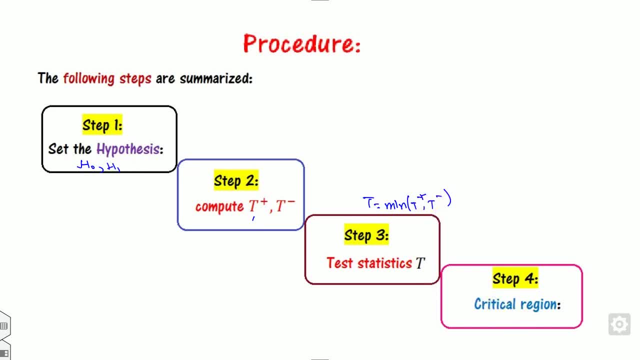 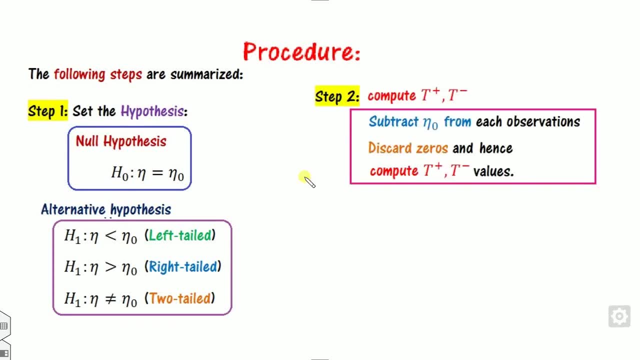 negative and we will see about the critical reason. Okay, so the hypothesis H0 is always the equality alternative is any one of them. Step 2 is compute T positive. How you compute them: You can subtract eta 0 from each observation and after that you can subtract eta 0 from each. 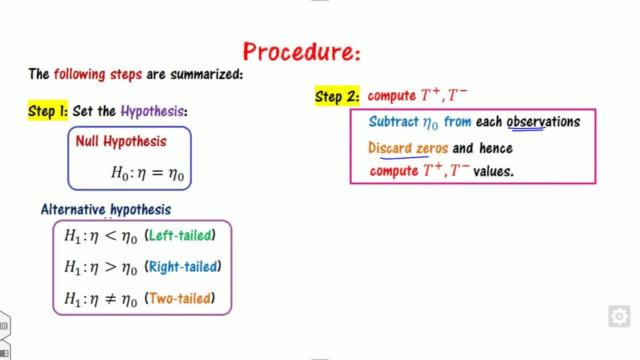 observation and after discarding the zeros, we will compute T positive and T negative. Then we will step third. that is the test statistics. we will calculate here and the critical value is defined as here. So let us discuss with some example Where. what is that? Tc is Where? 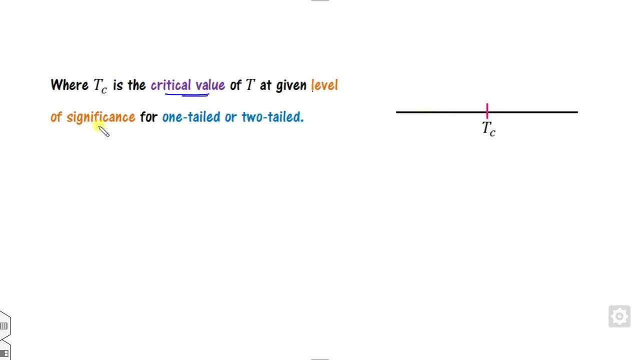 Tc is value of the critical value at the given level of the significance. So if this is my value, which is obtained from the table, so then the critical reason is my T less than equal to Tc. This is my critical reason. So if any value, if any value lies here, it means 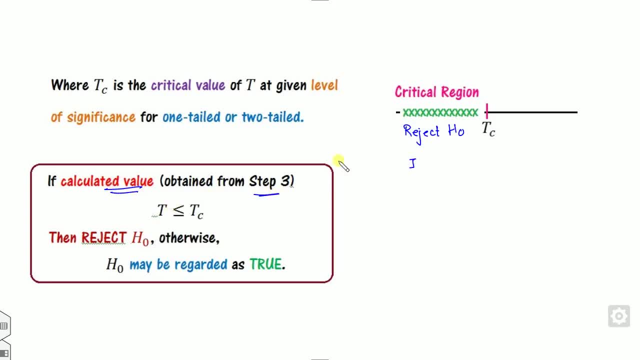 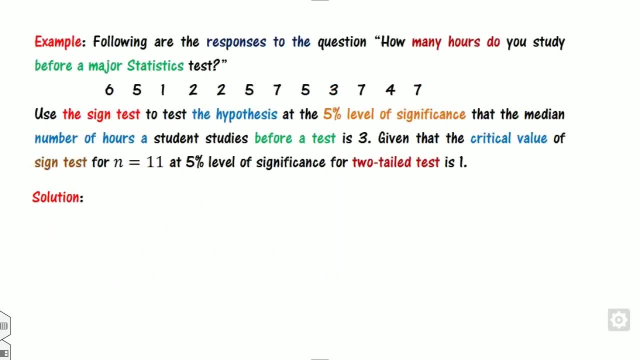 if the calculated value- that is a step third- is- lies here, we will reject H0.. If it lies here, we will. we may be regarded as a accepted H0.. Look at the examples to explain this. So say: following are the responses of the questions: How many hours do you study before? 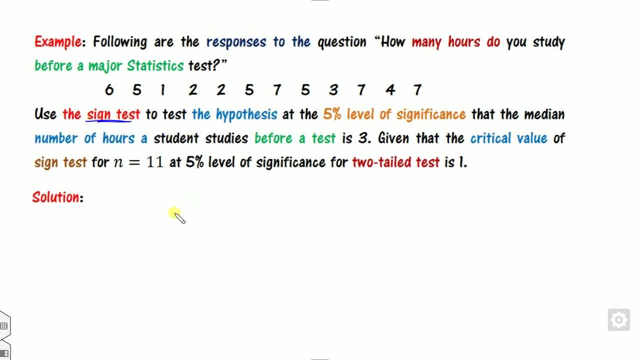 the major statistics test Using the sign test. so what is the step? number one? You have to define the H0 and H1. So what is the question? is that, what do you want to compute? The median of the students before the test is 3.. So 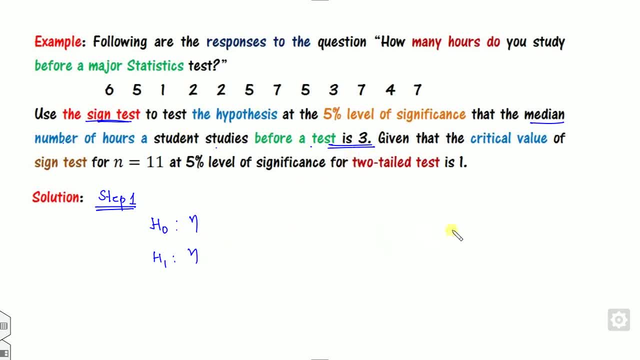 the median median is, eta is 3, that is equality. So whenever there is a equality we always define as a H0. So this is not equal to 3.. So it means this is my total, So the sample. 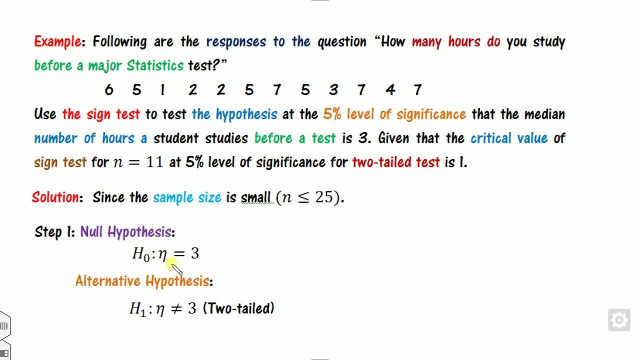 size n is small, So we will call as this sample size, So H0s. So this is a two-tail. What is the step two is We will subtract this 3 from each of the numbers. So what is? the first number is 6 minus 3, that is a positive. 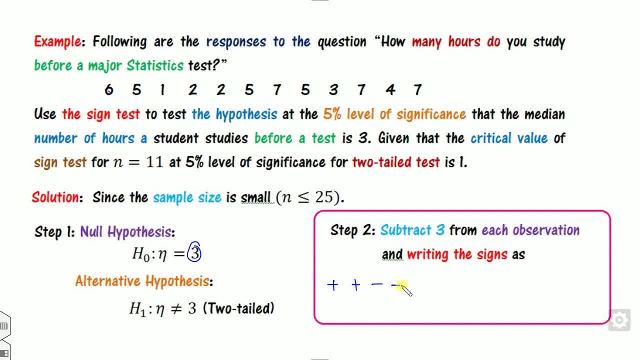 5 minus 3, again positive. 1 is a negative, Then 2 is a negative, and so on. We will calculate as here. Then we will calculate the T positive and T negative. How many positives are there? 2,, 3,, 4, 5,, 6,, 7, 8.. 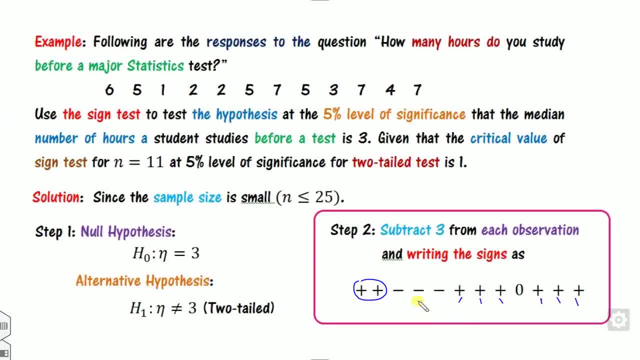 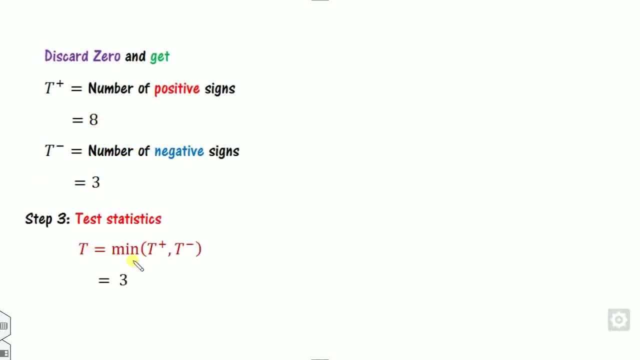 8 are my T positive? How many T negatives? 1,, 2,, 3.. So there are 3 T negatives. Then we will calculate the T as here. That is a step 3.. Now, the main thing is a step 4.. So 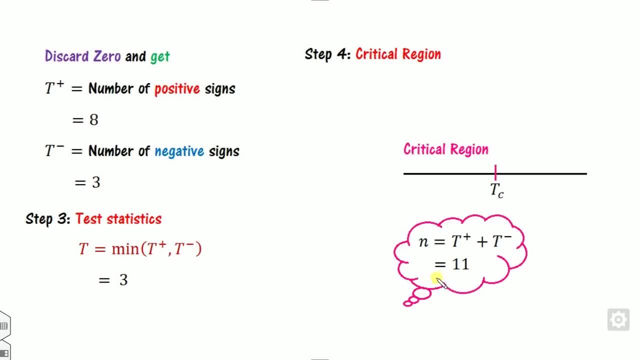 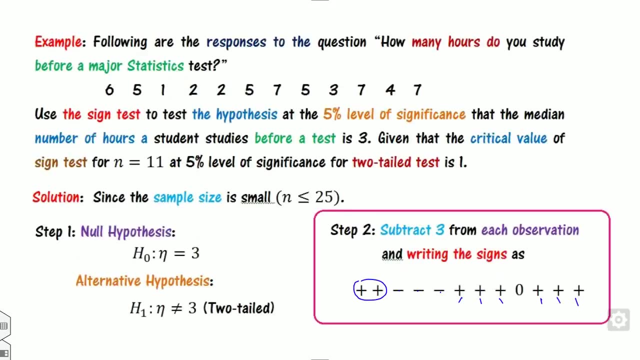 firstly calculate n T positive plus T negative, that is 11.. Now my task is to find the value of the Tc. So look at this given statement. It is given that the critical value for the sine test for n is equal to 1.. So this is the critical value for the sine test for n is equal to 1. So 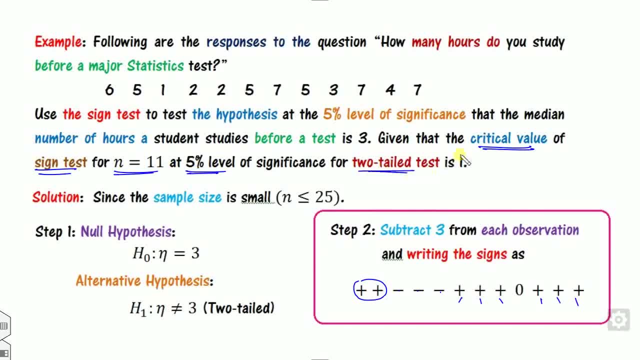 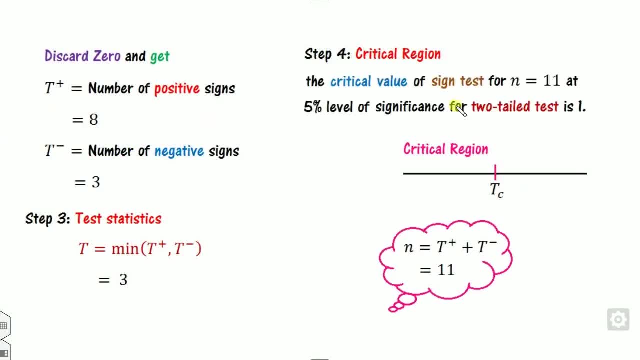 at 5, percentage level of significance for the 2 tail is 1.. So this is 1 is my critical value, for n is 11.. So this Tc is my 1.. So it is given. So this is here. So what is the meaning of this? 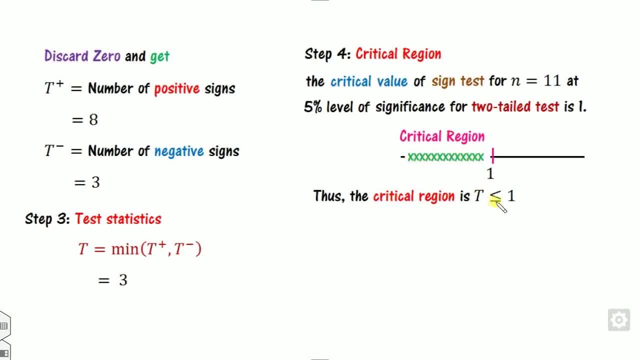 is. So the critical reason is here: T less than equal to 1.. Now check where it lies. This is my minus infinity to plus infinity. So where is 3 lies? It lies here, So look at that. 3. 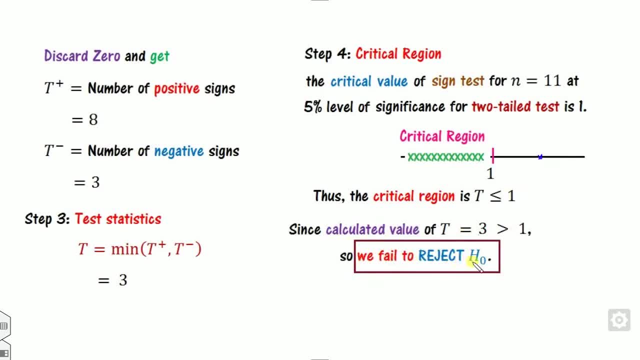 is greater than 1.. It lies here. So we fail to reject H0.. So what is your H0 is? Look at that eta is 3 and it is not equal to 3.. This is my reject H0.. This is accepted H0. It means this: 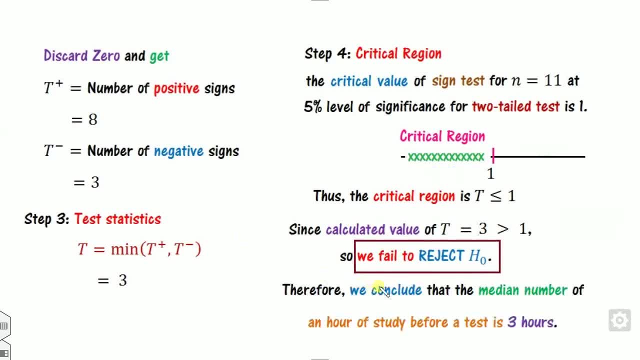 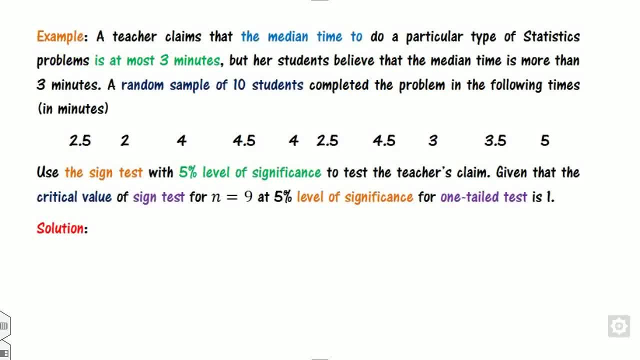 is accepted. So what your conclusion is? We conclude that the median number is 3.. So this is the way you can compute them. Look at the one more example So it will be clear to you. So, firstly, the sample size is very small. So n is my less than 25.. So 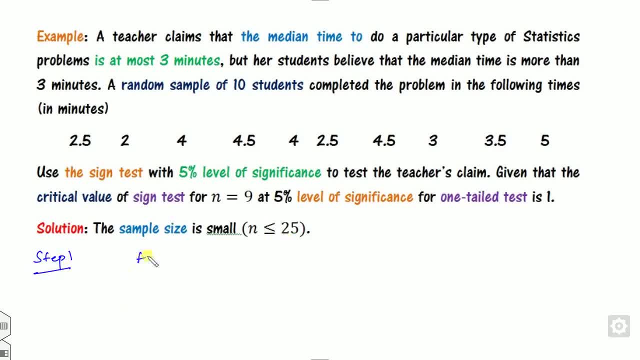 it is there. So define this step 1.. H0, H1.. So what is that? Use the sign test that teacher claims. So what is the teacher claim is A teacher claims that the median time. So 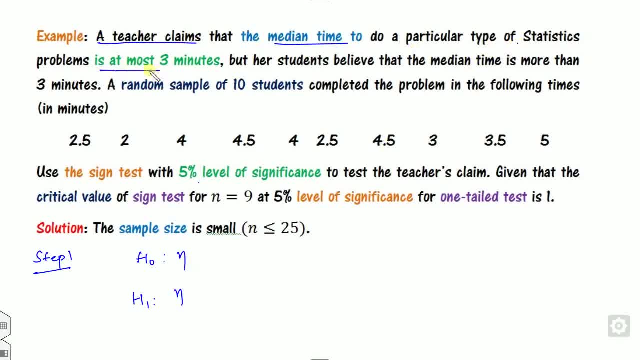 it is a median of the particular type- is at the most 3.. So it is not equality. So what is the meaning of the at most 3? It means less than equal to 3.. So it is not equality. So here this one. So what is the opposite of this is Here. So this is my. 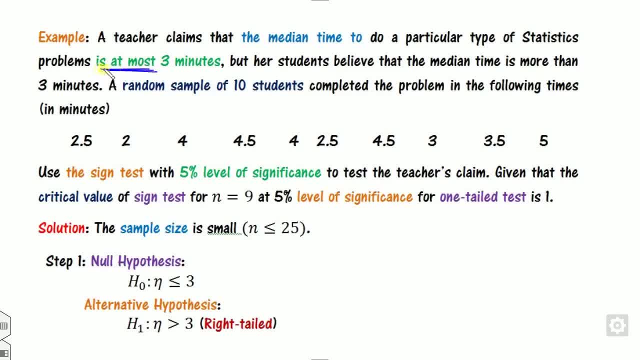 is at most. Sorry, this is less than, This is less than, and here is greater than, This is the at most 3.. So it is less than. So it is my left tail. So what is the step 2 is? You can subtract. 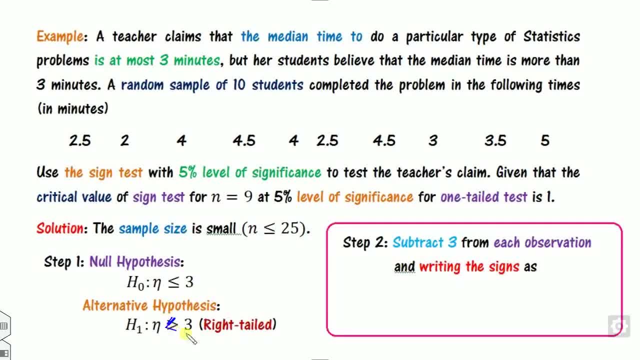 this 3 from each of the numbers. You can subtract this 3 from each of the numbers. So first one is negative, Second one: 2 minus 3 negative, 4 minus 3 positive, and so on. You will calculate. 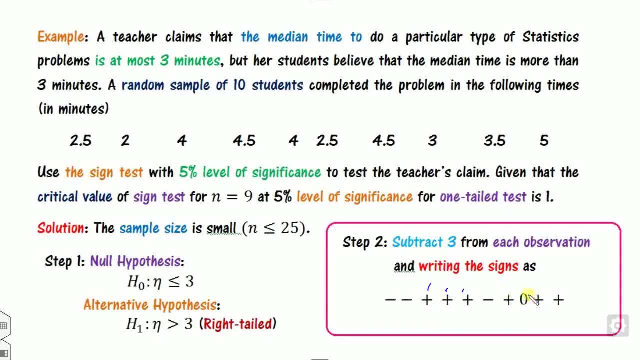 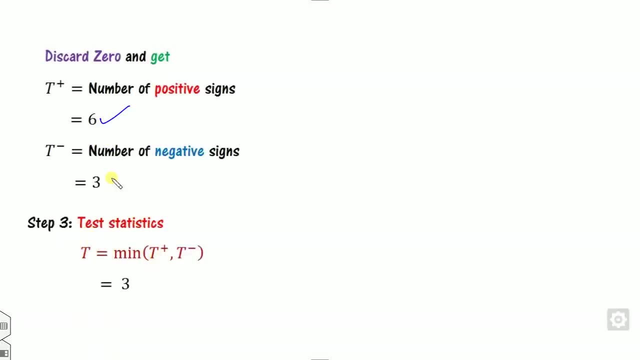 this. So how many positive numbers are there? Positive signs: 6 are my positive. How many negative are there? 1,, 2, 3.. So how many positive numbers are there? Positive signs? So t positive, 6, t negative, 3.. Then you have to find the capital, T Minimum of this. 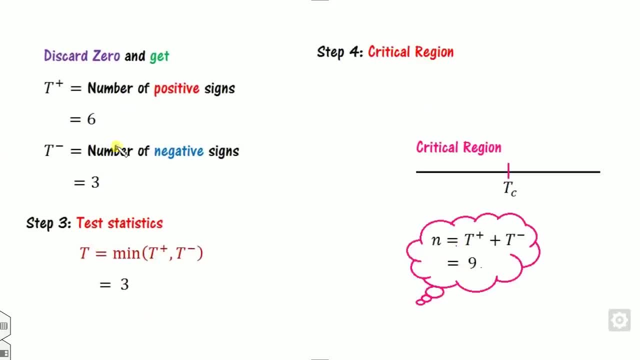 that is a 3.. Now you can calculate the n 6 plus 3, 9.. So you have to find here. So it is given that in the statement the sign test for the 9 degree of 9 at the 5 level. 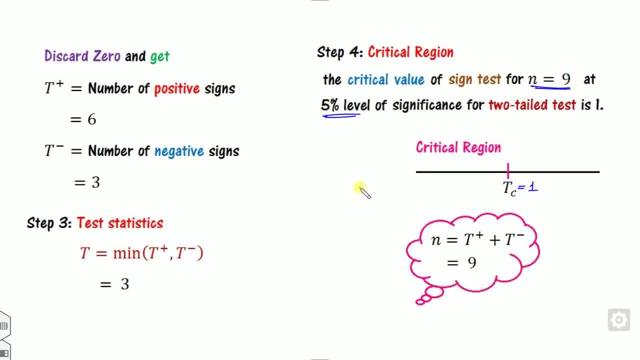 is 1.. So this value is my 1.. So the critical reason is less than equal to this 1. Critical reason is here, So this portion is my rejected H0.. This is my accepted H0.. So look at that, the value. 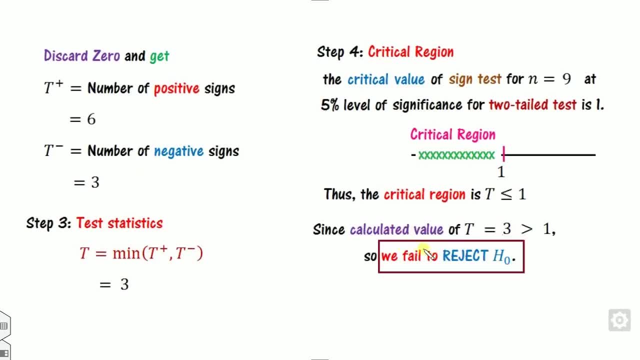 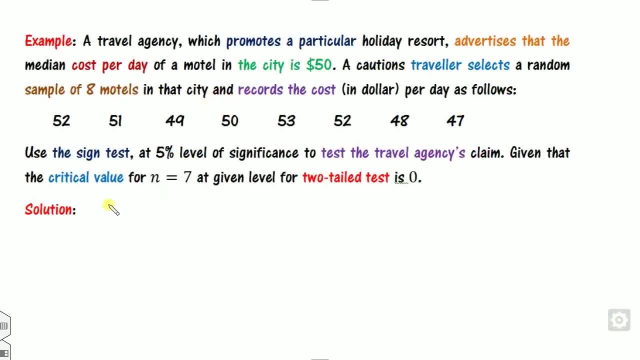 of 3 lies here. So this is greater than 1.. So we fail to reject H0 again. Hence we conclude that the teacher claim is, at most, is true. Look at one more example which will explain you more. So, firstly, again, the sample size is less than 1, or less than 25.. 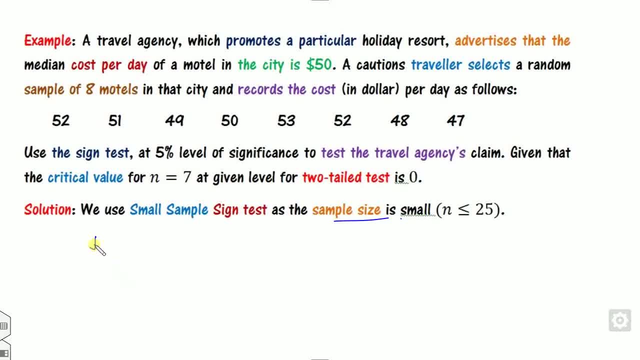 So we will use the small. So what is the H0 and H1?? So what is that The travel claim? So what is the travel claim? is A travel agency who promote a particular holiday advertised that the median cost in? 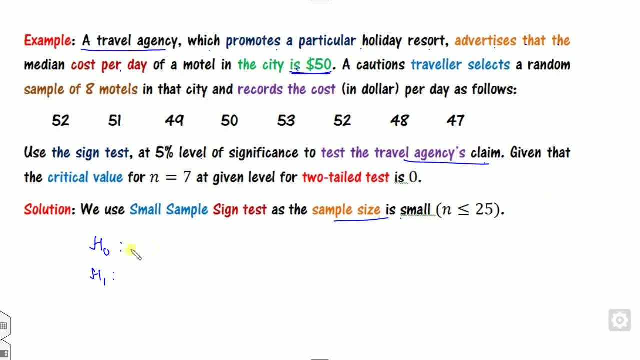 the city is 50. So this is is means equality. Okay, the task is 50. So, since it is equality, so that's why this is H0 instead of the H1.. So what is the opposite of this is Not. 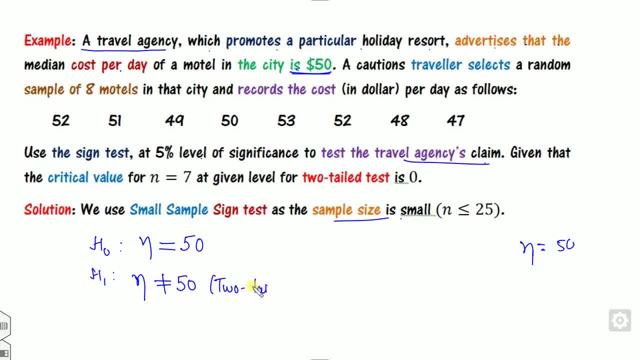 equal to 50. So it means this is my total. So once you are defining this, H step 1, what is the step 2 is you can subtract 50 from the each number. First number is my positive. Second is positive: 49 minus 50 negative. 50 minus 50: 0, 53 is a positive, then positive. 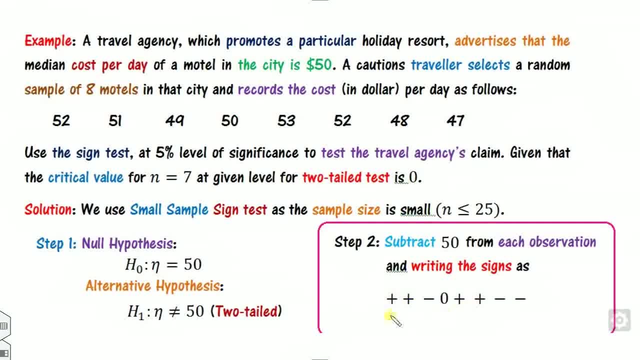 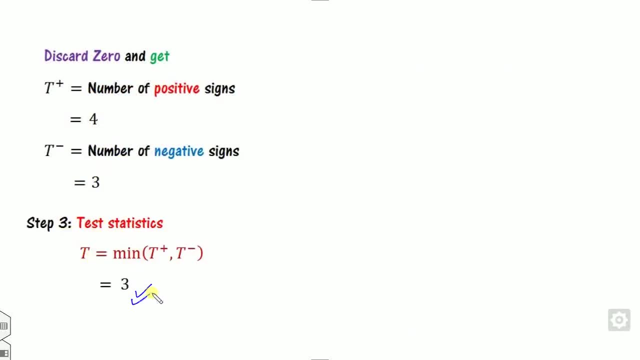 then negative, then negative. So you will calculate this one. So what is your T positive? 4. What is your T negative? How many negative numbers are there 3. So you have to define this. Calculate the capital T as a minimum of 4 and 3. Then what is the N is Step number. 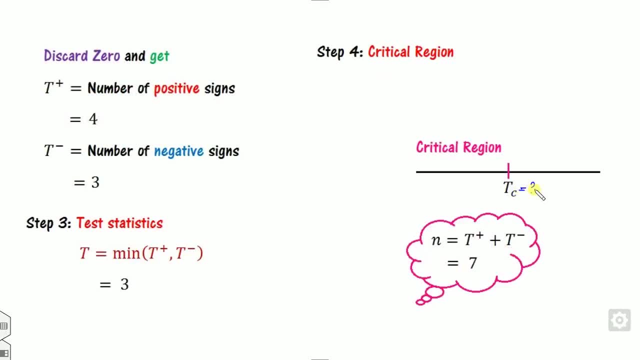 4, N is my 7. So you need this value. So it is given that in the statement the critical value for N is equal to 7 at 5 percentage level of significance for the 2 tail. Why it is a 2 tail? Look at the H1.. What is your H1 is? 1. What is your H1 is. 2. What is your H1 is. 2. What is your H1 is? 2. What is your H1 is? 3. What is your H1 is? 3. What is your H1 is? 3. What is your H1 is? 4.. So this is. 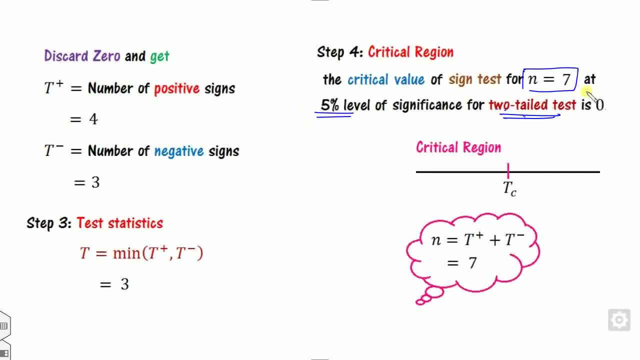 my H1.. So this is my Q1.. It is given as my 0.. So this value is my 0.. So, therefore, what is a critical reason? is this portion? So how you define that, this critical portion? 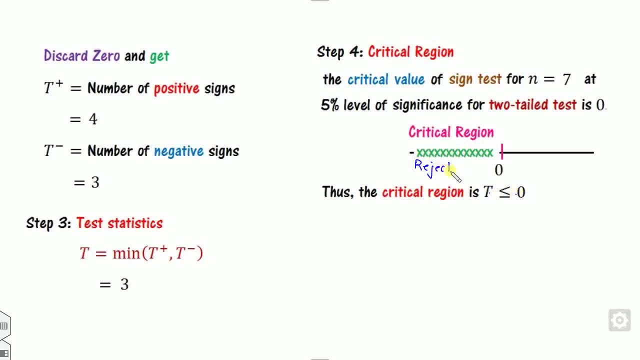 is less than equal to 0.. So this is my rejected H0.. This is my accepted H0.. So look at that where it lies. So, since it is 0. So 3 lies here, So we can say it is fail to reject. 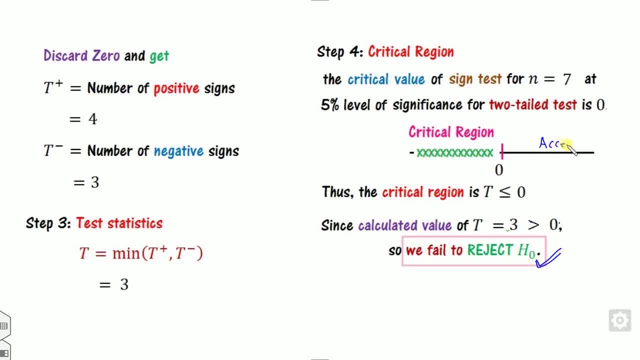 reject H0. fail to reject H0 means we will accept it. H0 and look at that. what is your H0 is median is 50 and so we fail to reject that is accepted H0. so this is accepted. so we conclude that the median may not differ from the 50. or you can say: the median of this is 50.. 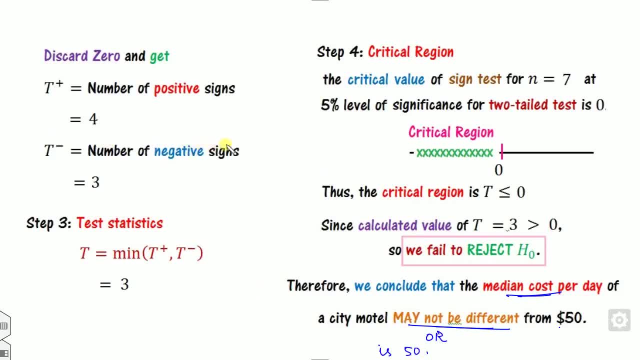 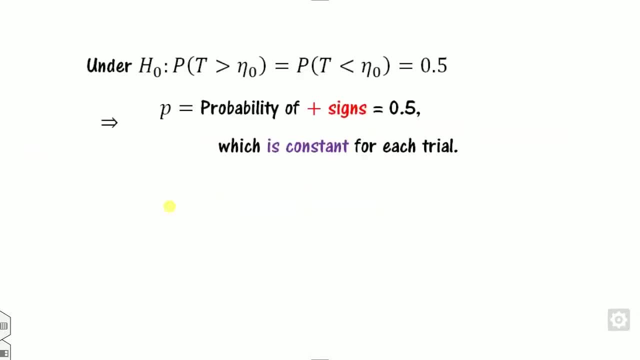 So this is a simple way you can solve the sign test. let us do for the large sample: what will happen when sample size is greater than 25.. So this is the definition of the median. so this P is nothing but the probability. so when we are talking about normal, when we are talking about 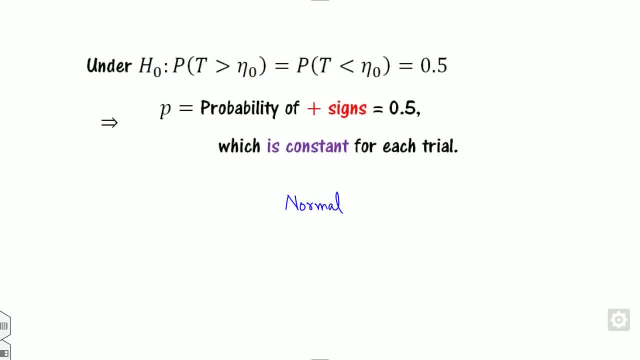 the large sample. so it means it is a normal distribution. so when it is a normal distribution, the probability is given as this. so the normal distributions is followed by the binomial distribution. so with parameter n and P here. so if T follows this, what is the mean of the? 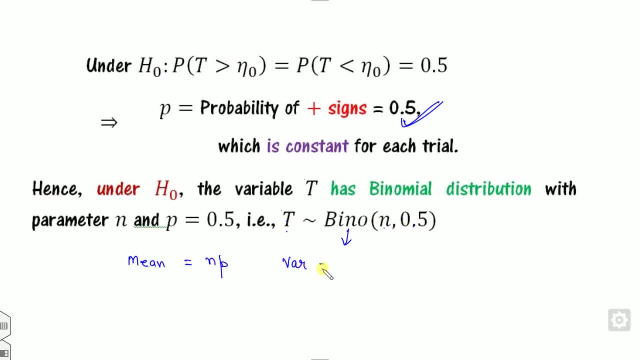 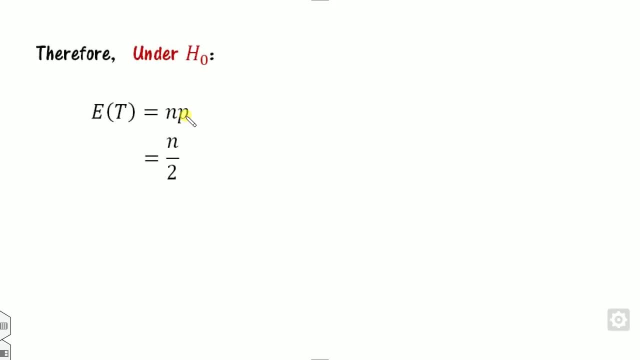 binomial distribution is np. what is the variance of the binomial distribution? is npq, so we can calculate that. so mean is np. P is my 0.5, so here variance is my npq. if P is my half, q is also half, so you can substitute here. this will here. so this is the 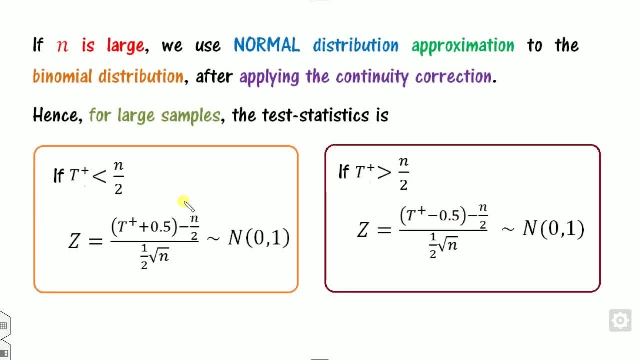 mean this is a variance. so by using the normal distribution we can apply here. if T positive less than of the half of the sample, we will apply z test as T positive plus 0.5, because this is the binomial is my discrete distribution, and we will apply the continuity correction by using 0.5. if 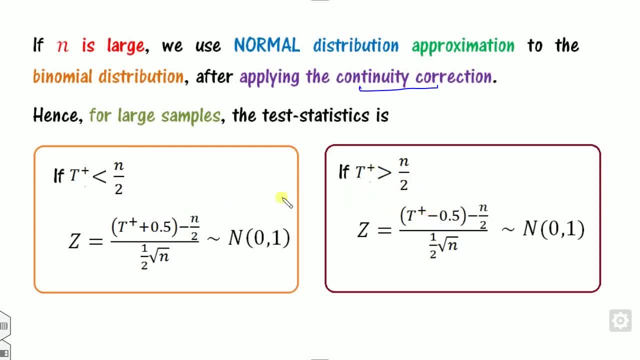 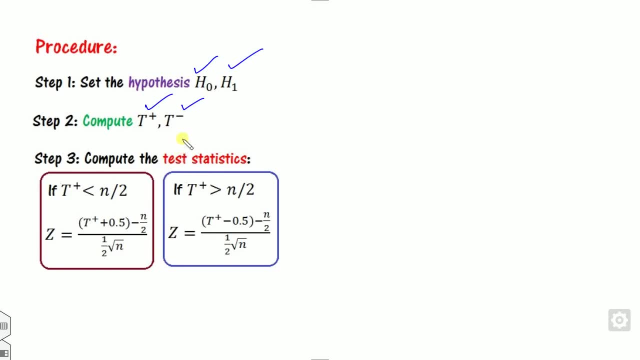 this is greater than n by 2, then we will use as a negative. so the working rules are same. we will define the h0 and h1. we will compute the value of the binomial distribution by using the continuity correction. we will compute at T positive and T negative. if T positive less than n by 2, we compute. 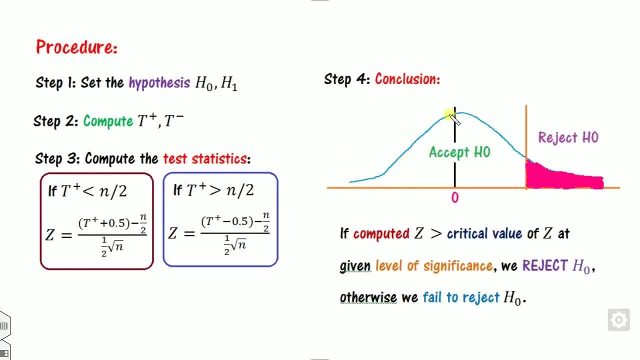 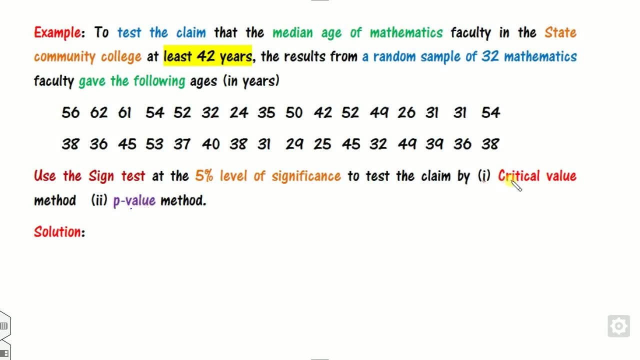 z as here. otherwise this, and since it is a normal distribution, we will draw the graph. this is the critical value and we will reject or accept the h0. look at this. so, since it's a normal distribution, so we will apply the P value as well as critical value, both. so firstly, look at that. the sample size. 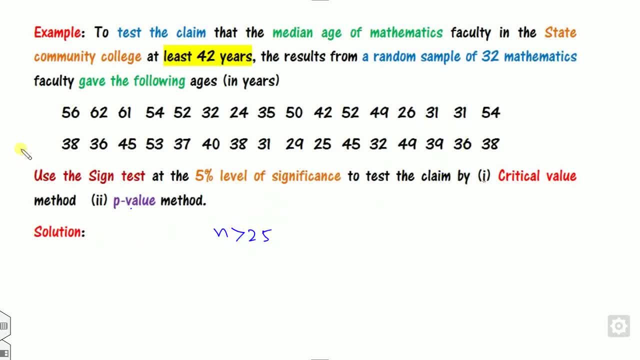 is greater than of the 25.. So firstly, define h0. so what is the claim? you can read: the statement is: at least 42. at least 42 is not the equality, how you write that this is so it is not equality. so you can write: 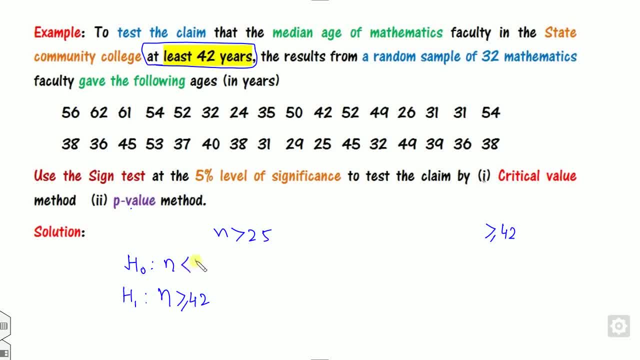 here as this. what is the opposite of this is less than so. this is my h0 and this is my h1. now you can define: subtract 42 from each of the observations. you can subtract 42 from each of the observation. look at the first number is positive. second number is positive. 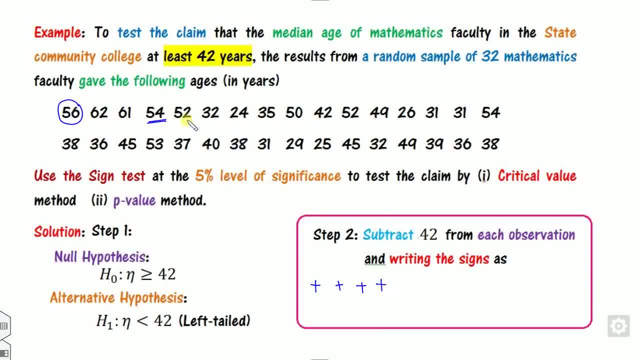 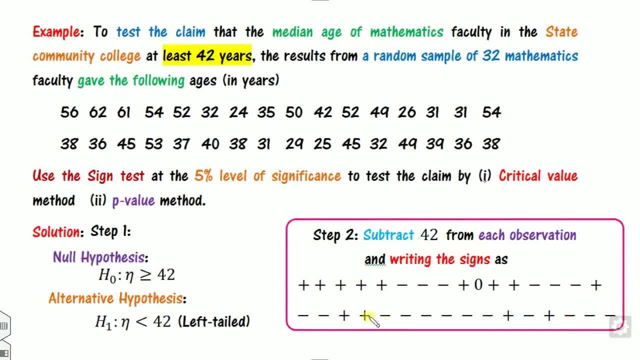 third is positive, fourth is again positive, fifth is again positive, sixth is my negative, and so on. so you can define like this: then compute the T positive and T negative, how many positive signs are there? one, two, three, four, five, six, seven, eight, nine, ten, eleven, twelve, thirteen? 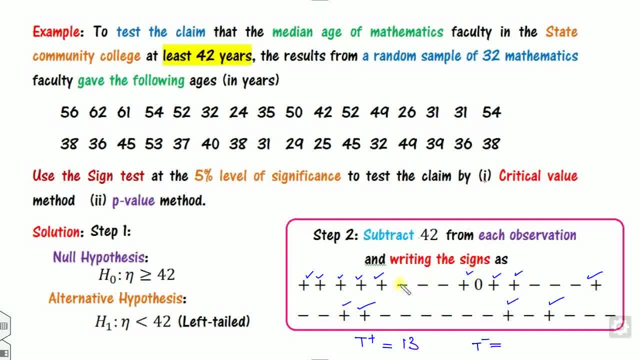 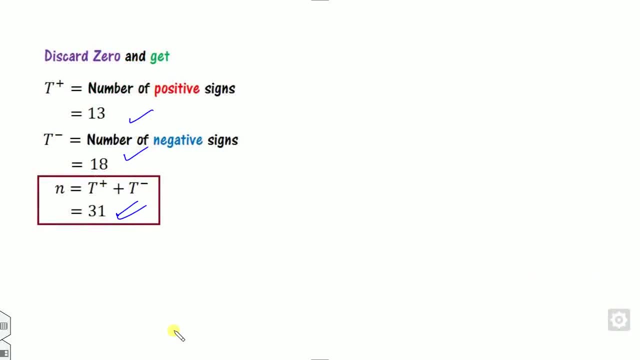 14, 15, 16, 17, 18.. here, okay, and how many negative are there? you can count them: 1, 2, 3, 4, 5, 6, 7, 8, 9, 10, 11, 12, 13, 14, 15, 16, 17, 18. so you can see T positive here and N is my 31.. 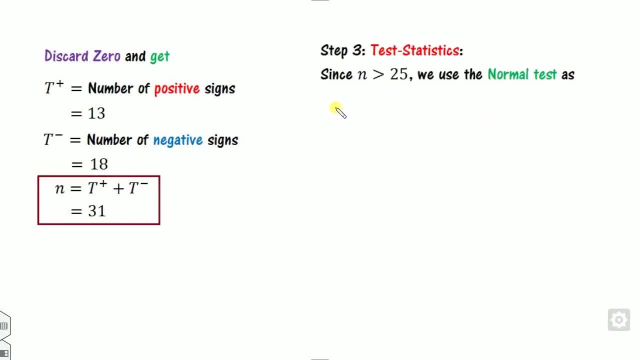 now, since, look at that N is my greater than or equal to 25, so we will apply the large sample T positive greater than n by 2. so look at that T positive is 13. so whether 13, what is that 13, is less than of the 31.2, so this satisfied. so, since it is this, so we will apply here. 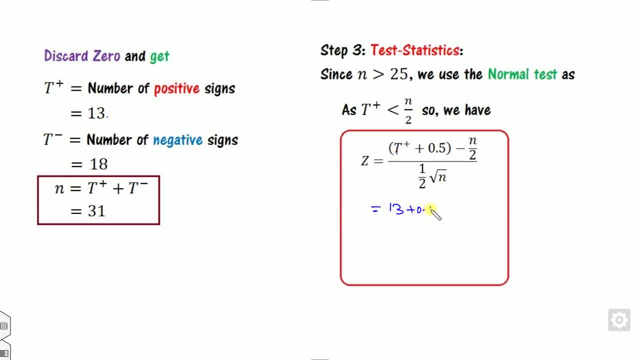 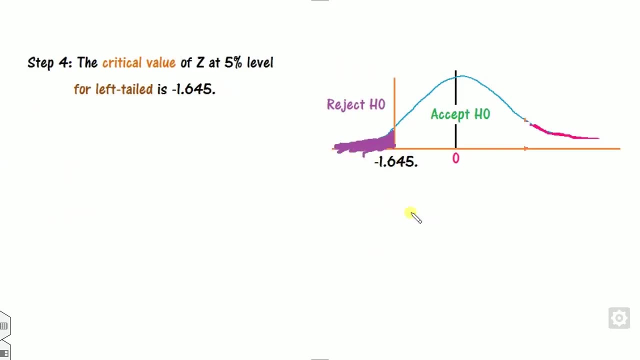 what is the T? positive is 13 plus 0.5. what is the n is 31 by 2 divided by half of 31. so after solving this you will get here. so this is step third. now in the step 4. so what is your? this is a negative, so it's a left tail. so the critical value at the 5 percentage: 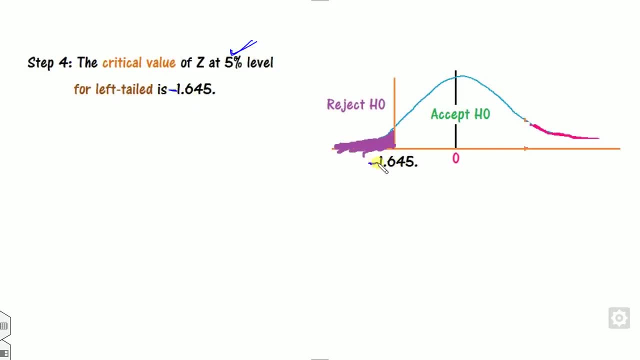 level of significance is minus 1.645. so look at that. the value is minus 0.718. where it lies? it lies here, it lies in the accepted H0. so since it here, so we fail to reject H0. hence the claim of the median test, at least, because what is your H0 is at least 42, and 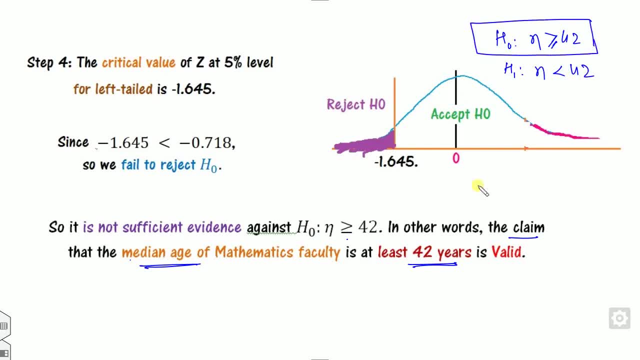 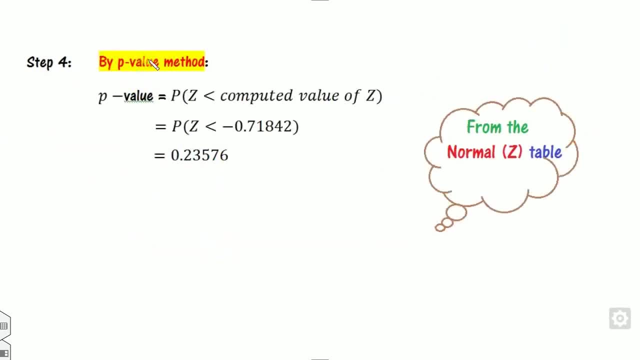 this is here, so this is accepted, so at least is valid. look at one more example. okay, how to calculate this. compute by P value instead of this. step 4, if you want to calculate the P value, So look at that. what is your H0 is: 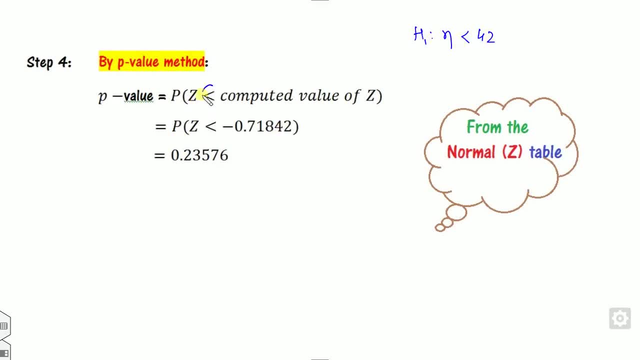 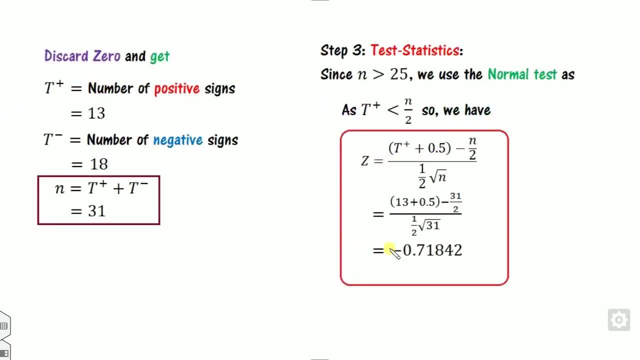 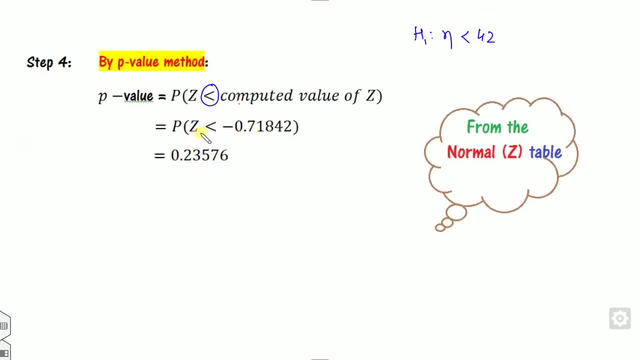 Less than of the 42, say left tail. so that's why this sign is less than what is the value of the Z we computed as. look at that, the value of the Z we computed as this number, so we will write the value of computed here. so the value of this you can see from the normal. 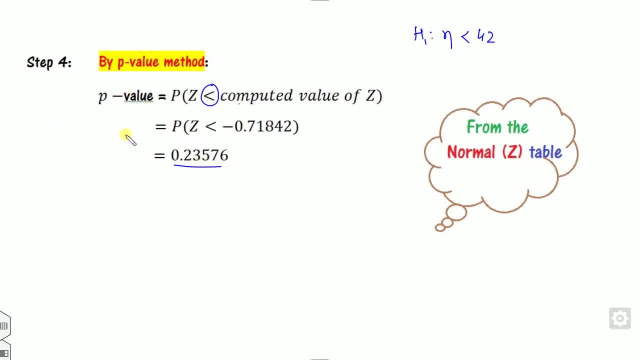 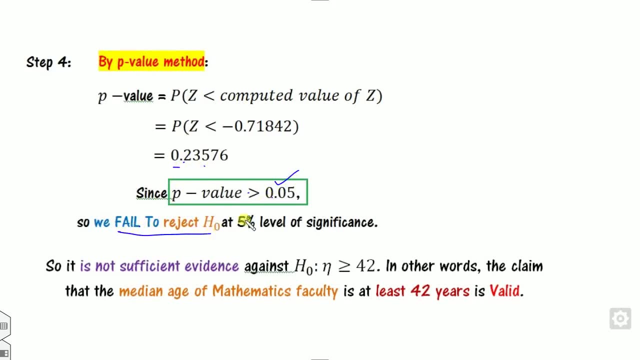 distribution table you will find here now. since the level of significance here is 5 percentage and this value is greater than 5, so we will fail to reject H0.. If P value less than of the level of significance, we reject H0. if P value greater than of the: 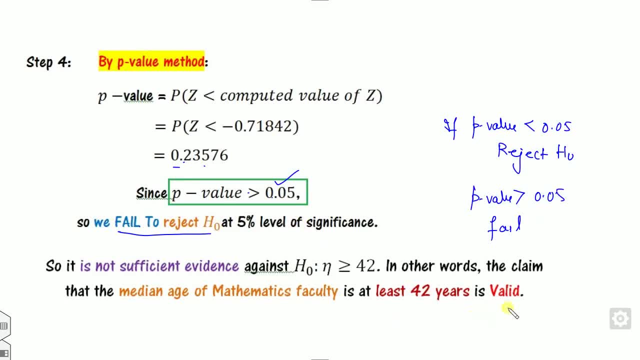 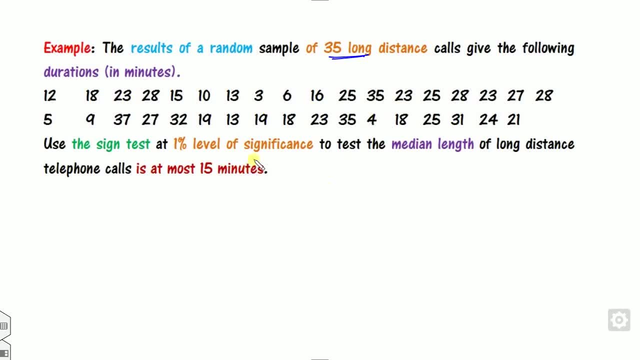 0.05. we fail to reject H0. so the claim is valid. look at one more example. so there are the 35 numbers are there? so definitely it's a large sample test. so what is the H0 and H1.. So the H1 is the median median, that's the eta, at most 15. so you have to define as at: 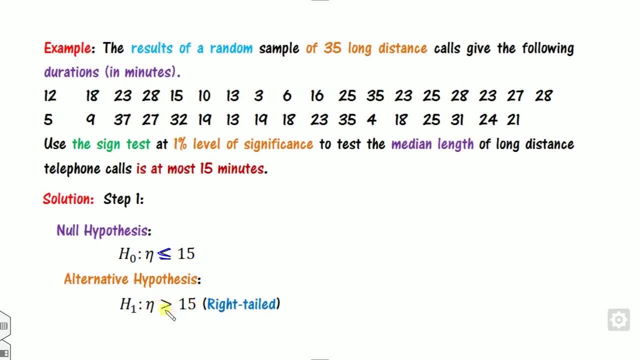 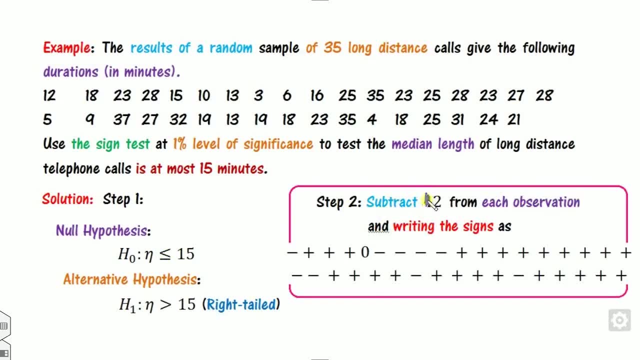 most 15. that's a less than equal to is at most and here. so it's a right tail. so step 2 is: subtract this 15 from each of the sorry, subtract 15 from each of the observation, so you will get the first number as a negative, second number as a positive, third is positive. 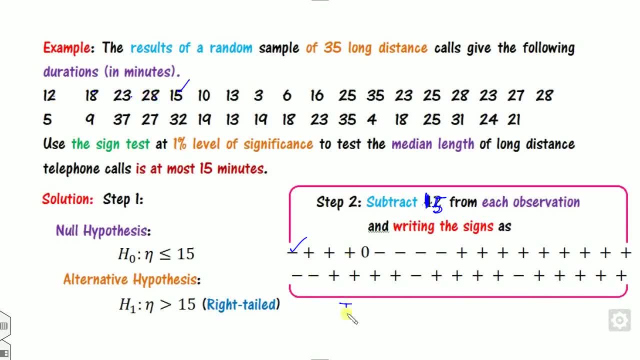 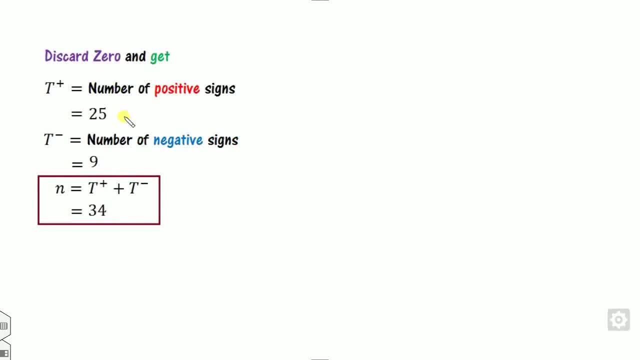 fourth positive, this is 0 and so on. Now you will calculate the T positive, How many positive numbers are there signs, and how many negative signs are there? you will get 25 and 9. you will get here then, since here. so we will check whether the T positive. 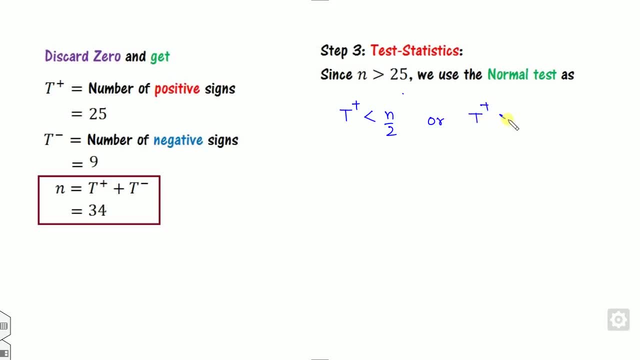 is less than n by 2 or T positive greater than n by 2, which one satisfy. this is 25 and by 2 is 17, so this satisfied. So we will calculate this value by using negative signs. Okay, So you will get as 2.57. now it's a right tail, so you have to write this one because 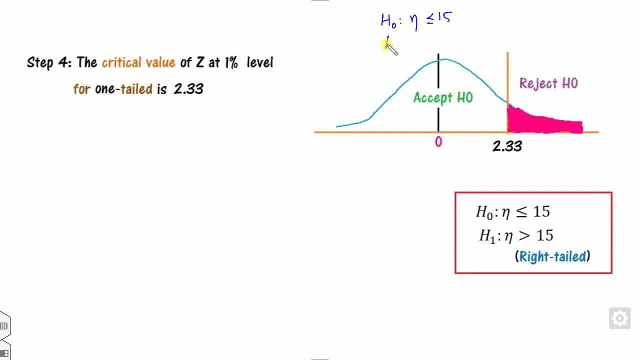 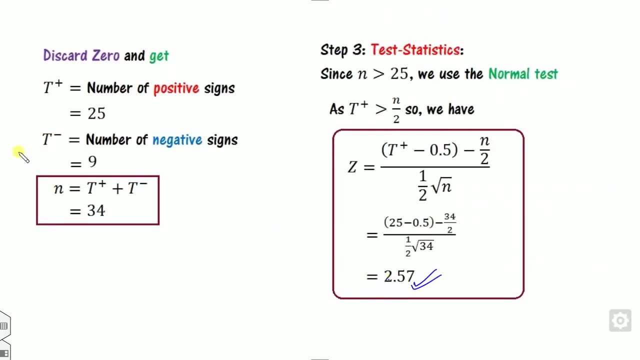 what is your H0? this is here. H1 is my right tail. look at that. this is right tail. so you have here. so the level of significance for the 1% level of significance is 2.33. okay, so what is the value of the Z is 2.57. where it lies? it lies here. look at this. this is. 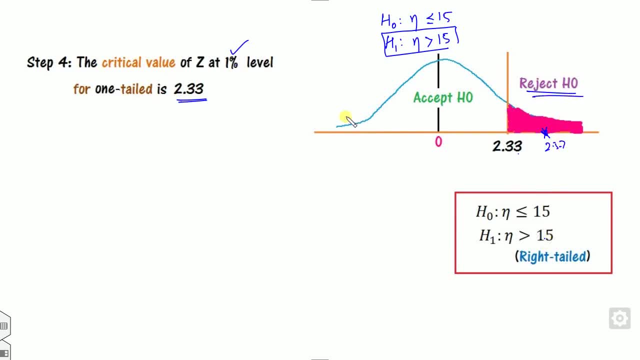 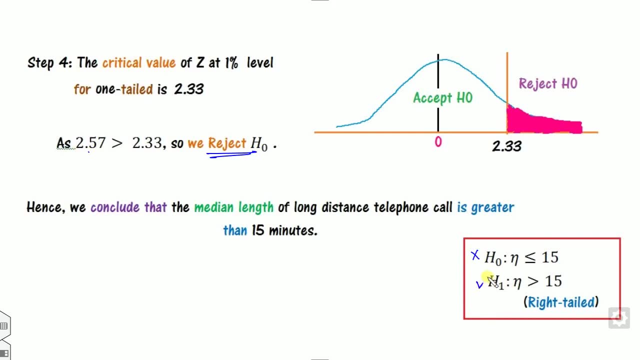 H0.. H1: 2.57 here, so it lies in the rejected portion. so we reject H0, so this is rejected. it means this is accepted. so the median length of the long distance telephone call is greater than 15 minutes. So this is a step 4 by using the critical value, if you want to use this by P value. so 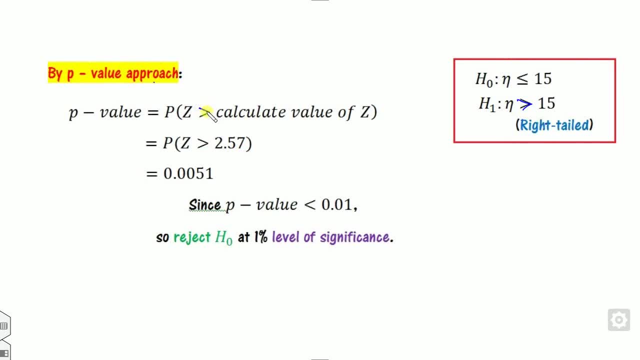 this is there. so this is a greater than sign right tail. so you have to use as a greater than. So what is the calculated value is a 2.56.. Look at the normal distribution table you will get. this level of significance is given. 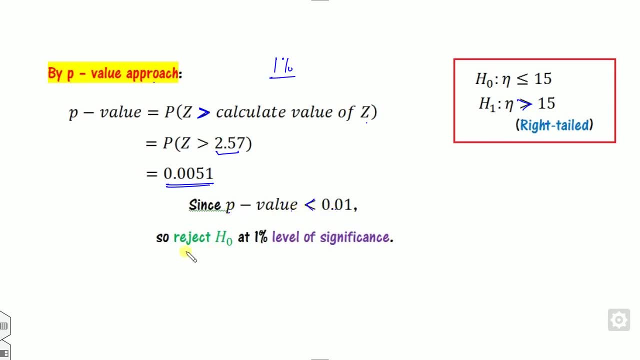 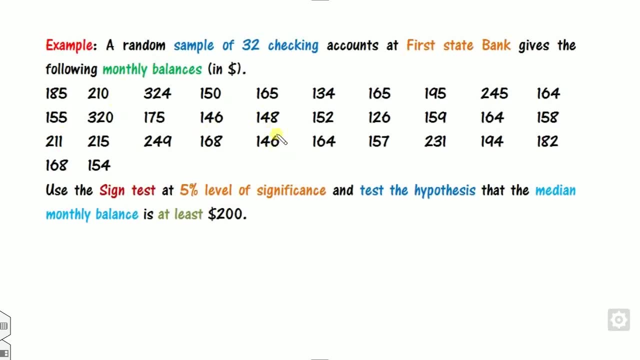 as a 1% is. so the P value is less than of the 1% is, so H0 is rejected again. Look at the last example. so again, these are the some informations. you firstly define the H0 and H1. that is the step. number 1 test the claim that the median monthly balance is at